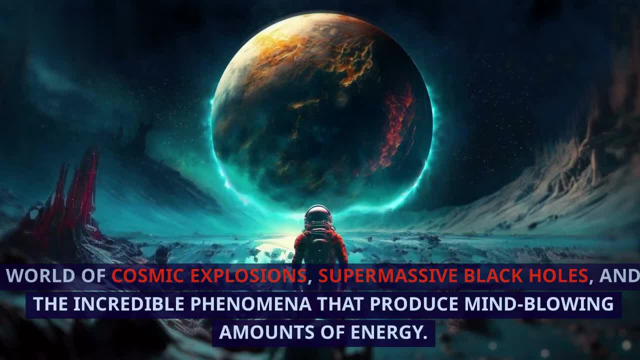 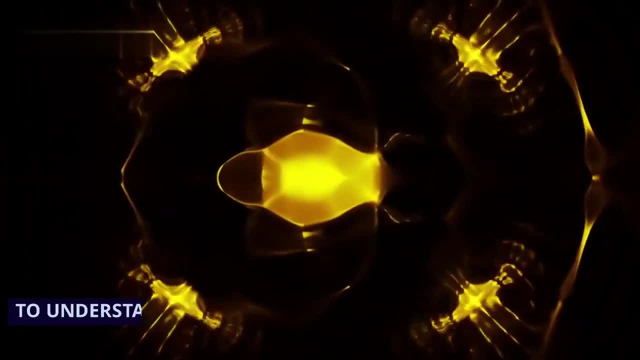 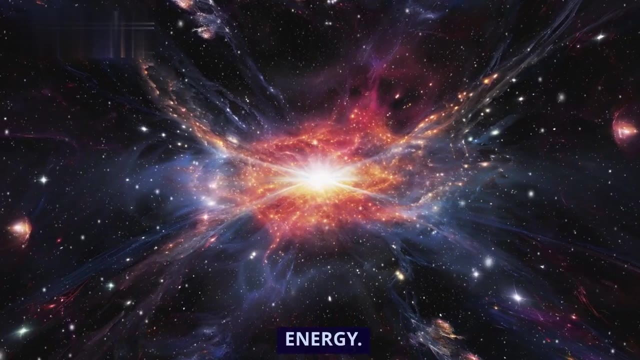 cosmic explosions, supermassive black holes and the incredible phenomena that produce mind-blowing amounts of energy. Buckle up as we unravel the mysteries of the cosmos To understand high-energy astrophysics. let's start with the basics. Our universe is a vast expanse filled with various forms of energy. 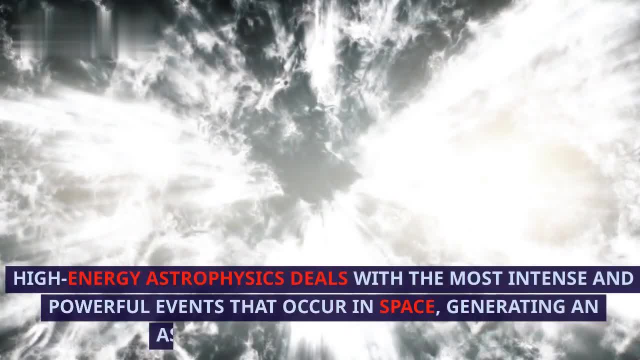 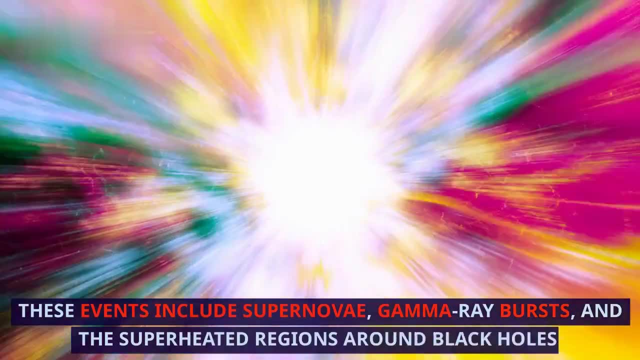 High-energy astrophysics deals with the most intense and powerful events that occur in space, generating an astonishing amount of energy. These events include supernovae, gamma-ray bursts and the superheated regions around black holes, One of the most explosive. 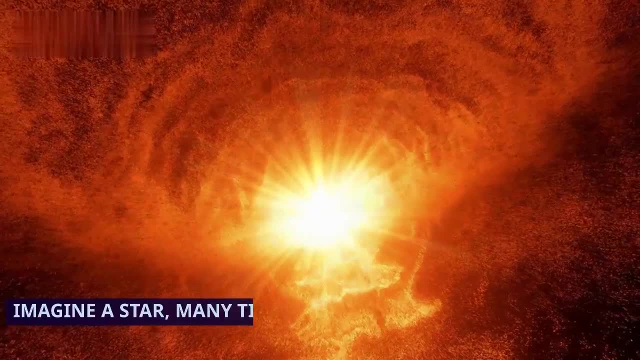 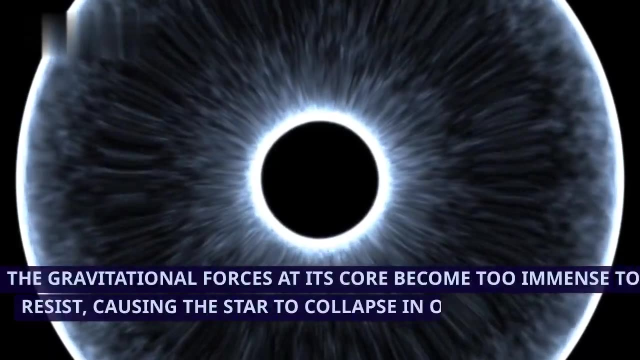 events in the cosmos is a supernova. Imagine a star many times larger than our sun reaching the end of its life. The gravitational forces at its core become too immense to resist, causing the star to collapse in on itself and then explode in a spectacular display of light and 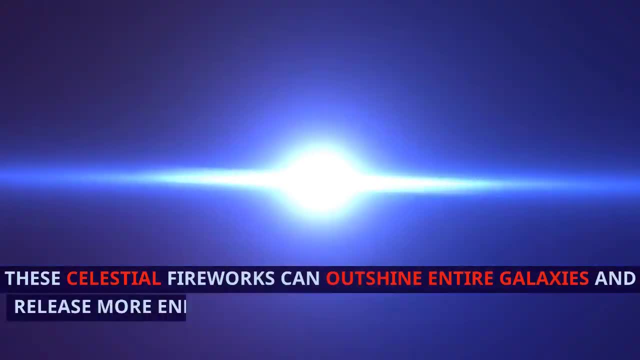 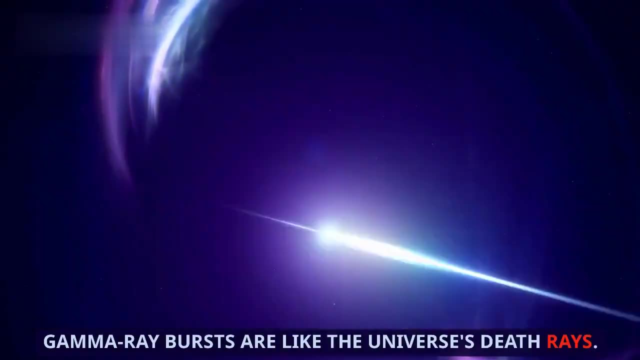 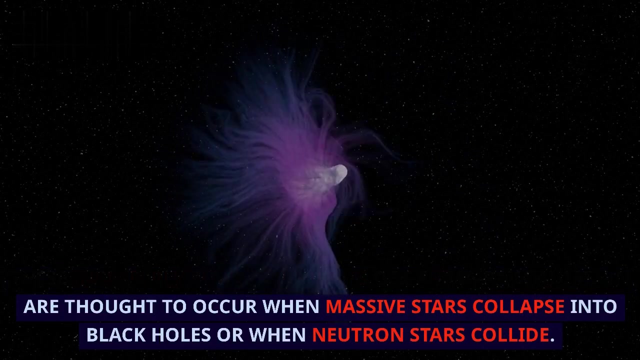 energy. These celestial fireworks can outshine entire galaxies and release more energy in seconds than our sun will emit in its entire lifetime. Gamma-ray bursts are like the universe's death rays. These incredibly powerful bursts of gamma-ray radiation are thought to occur when massive stars collapse into black holes or when neutron stars collide In a matter of seconds. 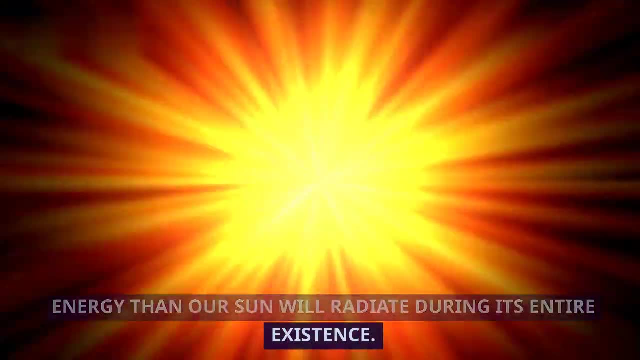 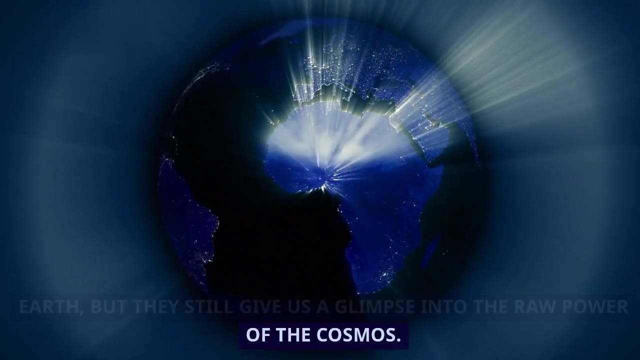 a gamma-ray burst can emit more energy than our sun will radiate during its entire existence. Fortunately, most of these bursts occur far away from Earth, but they still give us a glimpse into the raw power of the cosmos. Black holes are among the most mysterious and intriguing cosmic objects. 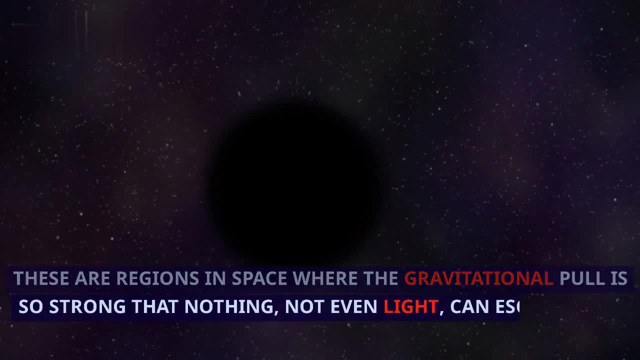 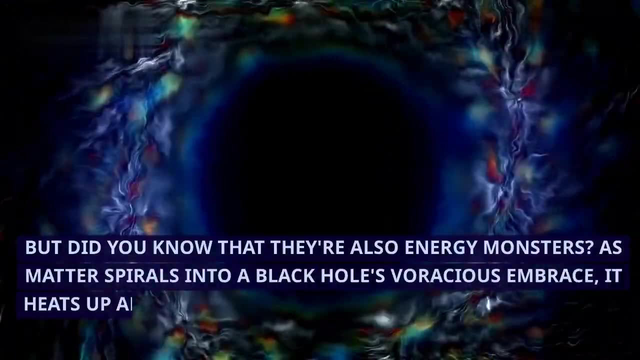 These are regions in space where the gravitational pull is so strong that nothing, not even light, can escape their clutches. But did you know that they're also energy monsters? As matter spirals into a black hole's voracious embrace, it heats up and releases tremendous. 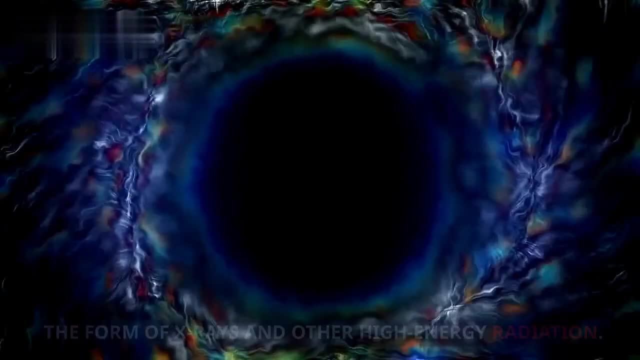 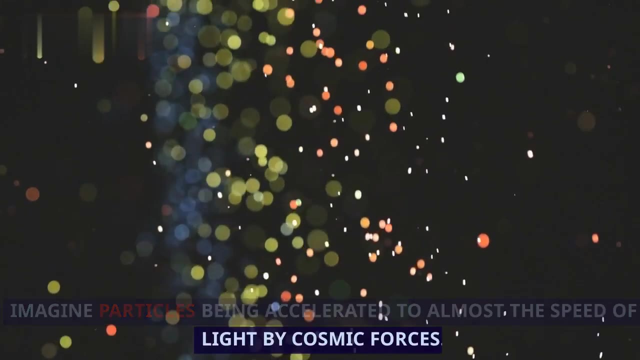 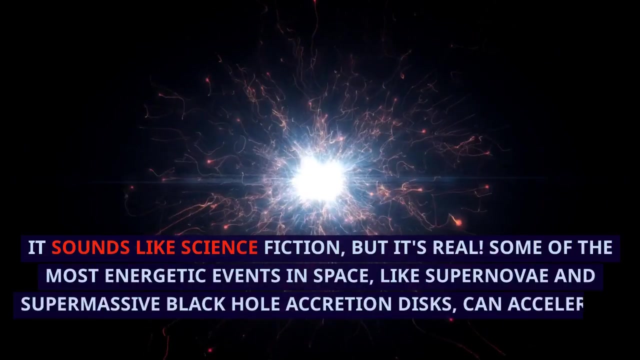 amounts of energy in the form of X-rays and other high-energy radiation. This process can light up the universe with cosmic fireworks. Imagine particles being accelerated to almost the speed of light by cosmic forces. It sounds like science fiction, but it's real. Some of the most energetic events in space, like supernovae and supermassive black, 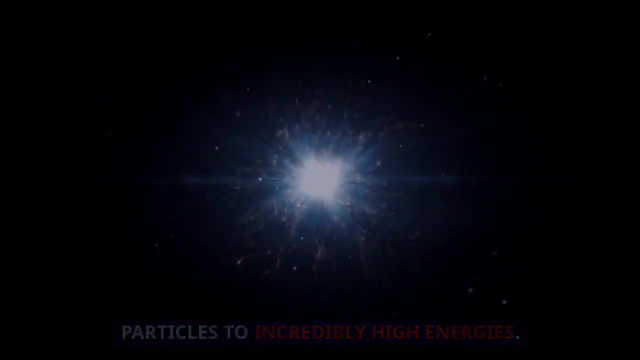 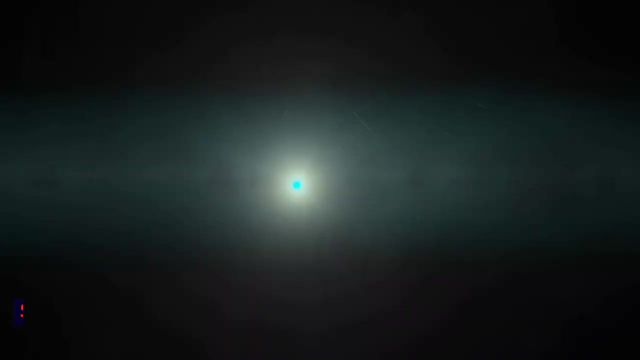 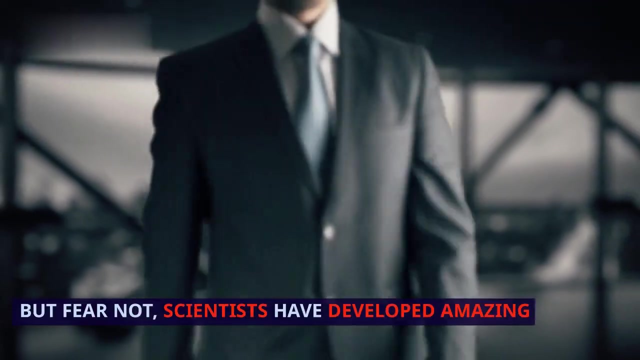 hole accretion disks can accelerate particles to incredibly high energies. These supercharged particles then zoom across the universe, creating cosmic rays that constantly rain down on Earth. Studying high-energy astrophysics isn't easy, as much of this is invisible to the human eye. But fear not: scientists have developed amazing tools to